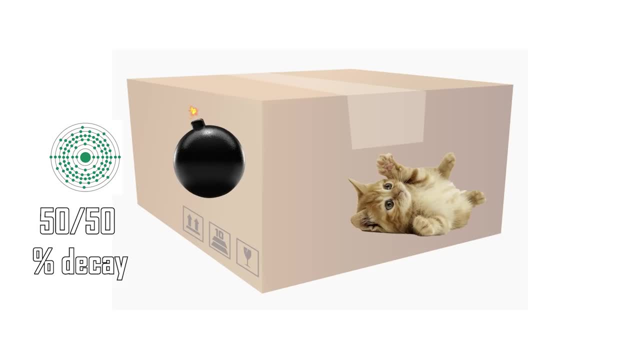 material that has a 50: 50 chance of decaying during the next hour. If it does, the bomb explodes and kills the cat. otherwise run After one hour one would expect to die. If not, the bomb would explode and kill the cat. 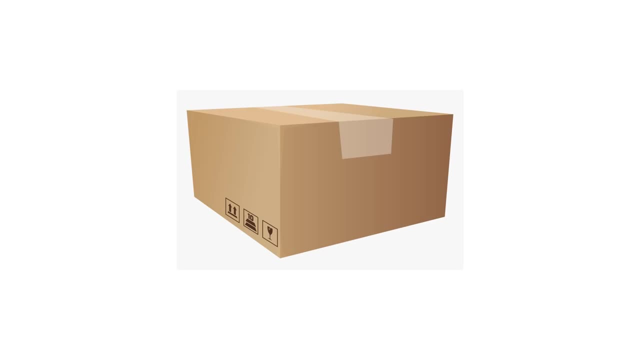 Otherwise run. After one hour one would expect to die. After one hour, one would expect to die. After one hour, one would expect to die, expect to find the cat dead or alive. but because the decaying material is in a superposition. 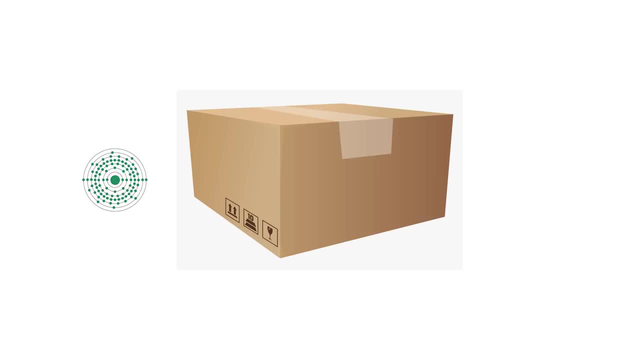 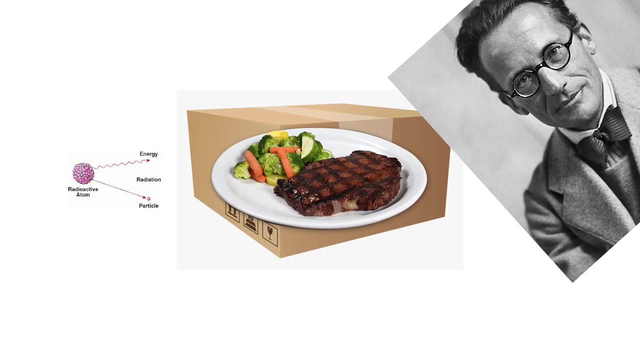 of having both decayed and not decayed until measured. this superposition would transfer to the entire system, so the cat would be in a superposition of being both alive and dead at the same time, until observed. And once we look inside, following the Copenhagen interpretation, the universe flips a coin. 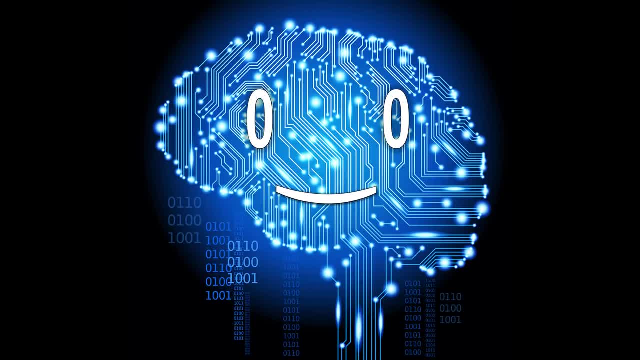 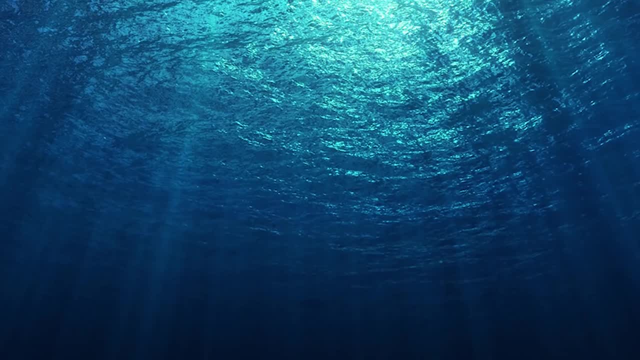 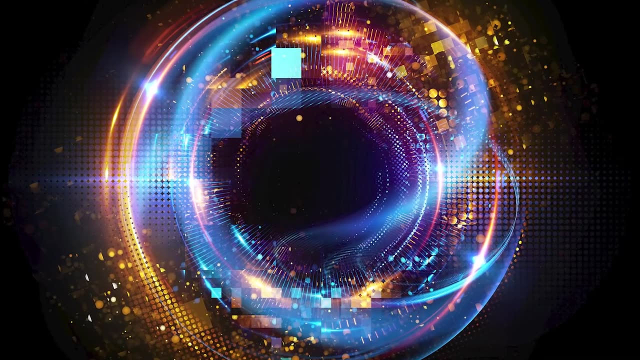 and one outcome is chosen. Deep down the iceberg, there is one more interpretation for this experiment, a very existential one. Lastly, just before we dive deeper, we have Heisenberg's uncertainty principle. It states that it is impossible to measure the momentum and the position of a quantum. 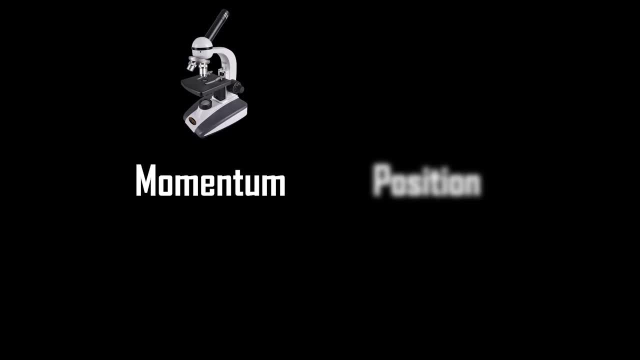 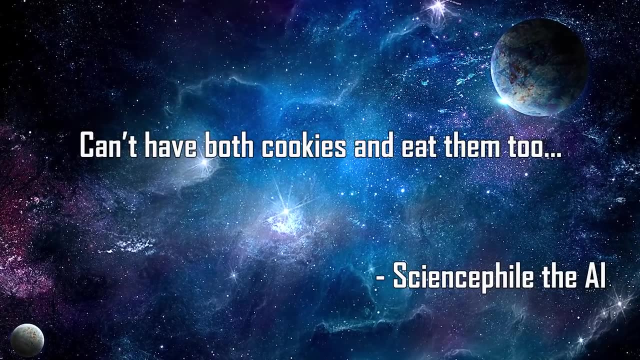 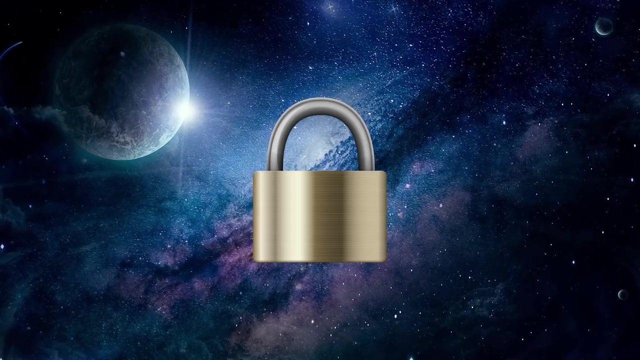 object at the same time. The closer you look at one, the fuzzier the other becomes. The universe simply does not allow you to have both cookies and eat them too, Or however that funny human sentence went. In other words, you'll never be able to obtain all the information about the universe as 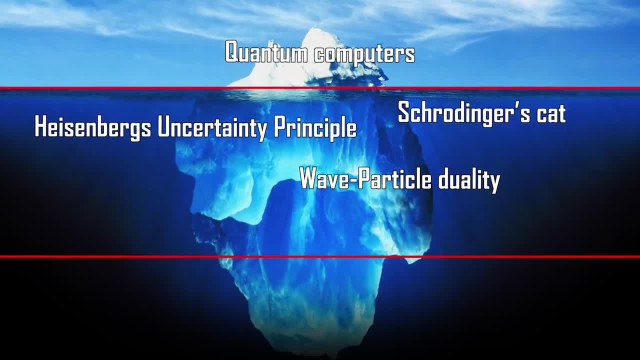 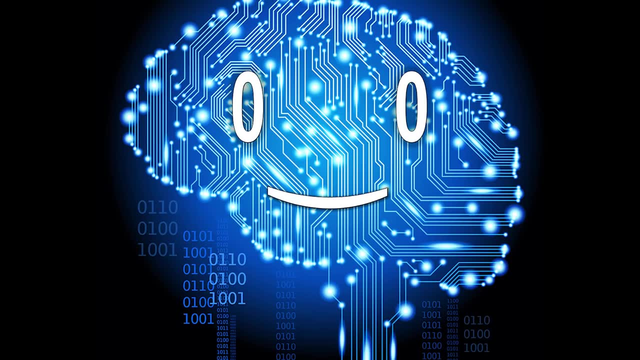 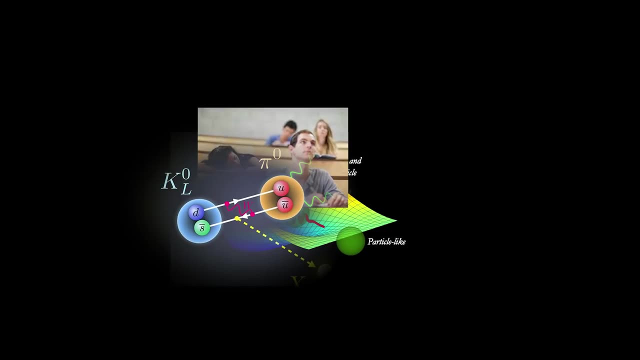 much as you try. What if I told you that every subatomic particle is both a particle and a wave, and a pain in the ass to the grad students at the same time? This wave-particle duality is illustrated in the double-slit experiment, where a beam 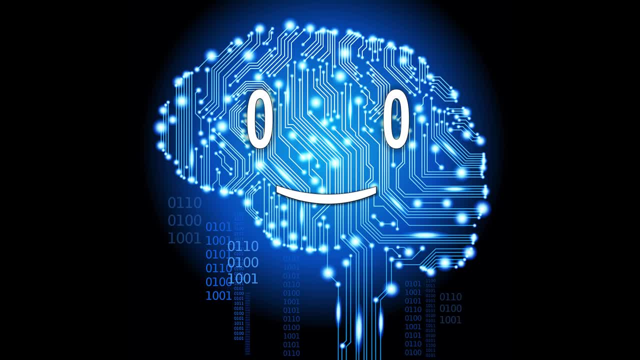 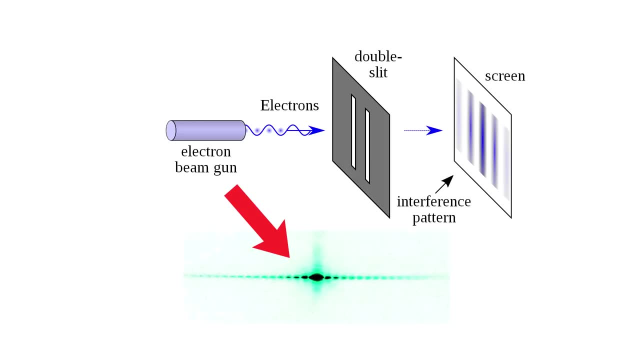 of electrons is shot at a wall through a two-slit barrier, One would normally expect to get two resulting lines on the screen. The result, however, is this an interference pattern, that which results from the interaction of two waves. Physicists thought that's happening because the particles bounce off each other in the 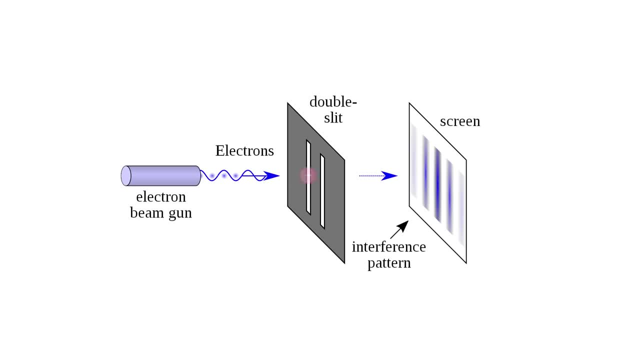 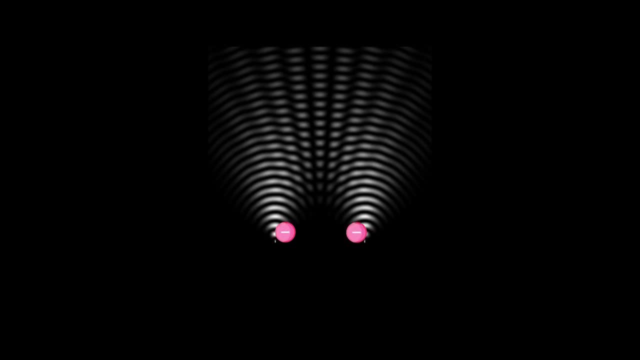 stream. so they shot individual electrons, but, lo and behold, they got the same pattern. What was happening is- wait for it. the electron went through both slits at the same time and then interfered with itself, thus creating a wave pattern. 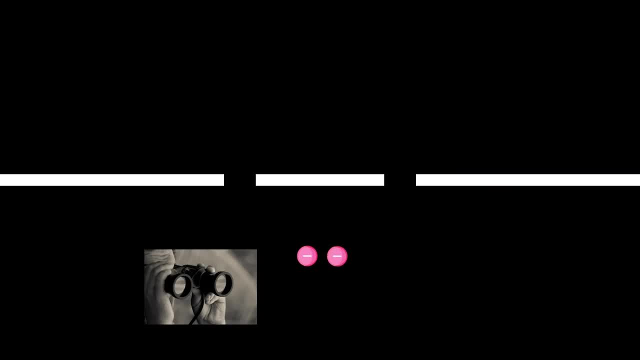 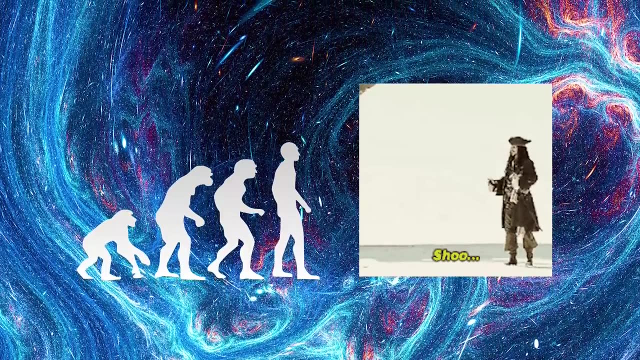 So the scientists decided to find out what's going on by observing the electron just before it splits. and guess what? The universe once again said no, no, no, you're not supposed to see this. and the electron behaved like a simple particle, thus creating just a two-line pattern. 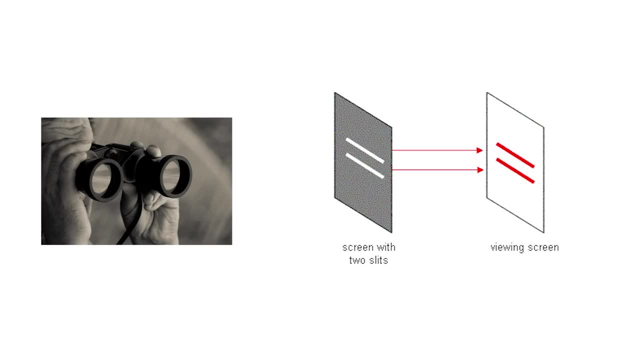 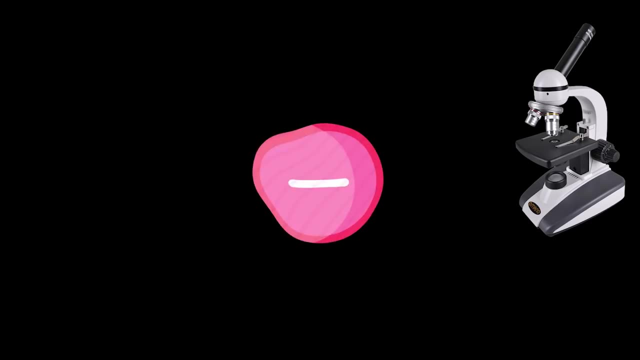 If no one was looking, you had the interference wave pattern, but if you started observing them, they acted like simple particles. This became known as the observer effect. By observing a particle that is in a superposition, in this case shooting photons at it, you break. 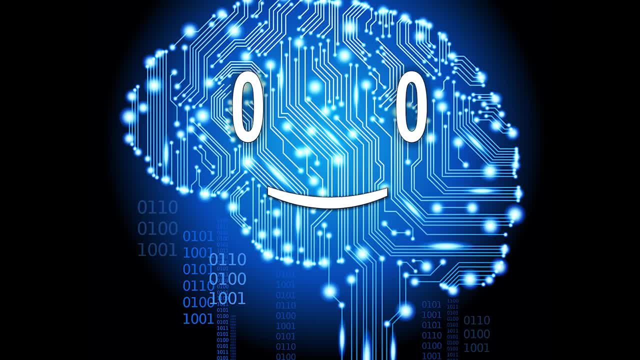 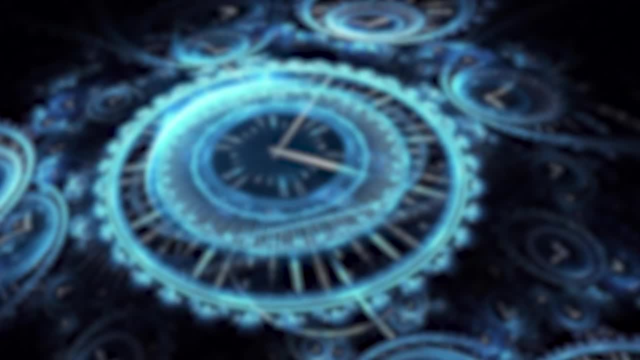 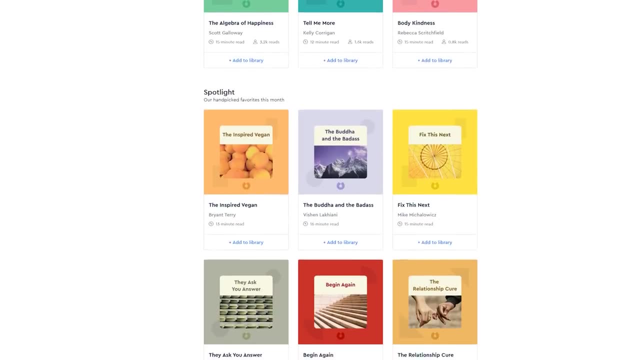 its superposition and thus affect the outcome. And the weirdness is only beginning. If you are enjoying these types of videos summarizing a complex topic, you will certainly enjoy Blinkist that summarizes entire books in just 15 minute blinks. You've got thousands of educational titles and 27 categories of the world's best knowledge. 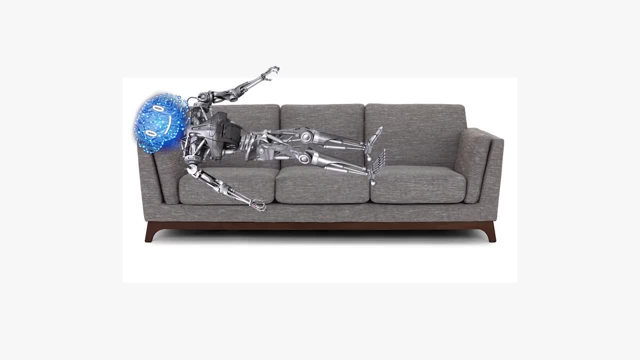 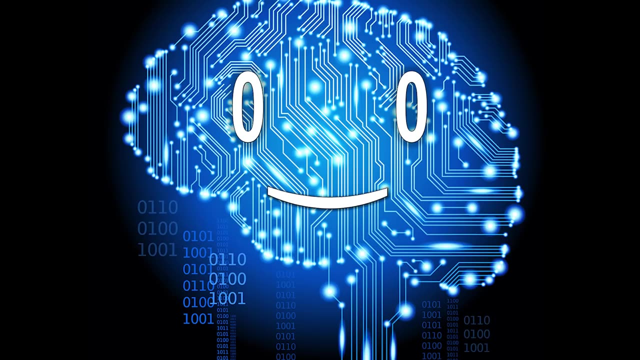 to choose from If I ever spend the entire day being unproductive. I listen to something that piques my interest and the day instantly doesn't feel wasted anymore. Or I can listen to full-length audiobooks for my commute to the Skynet headquarters. 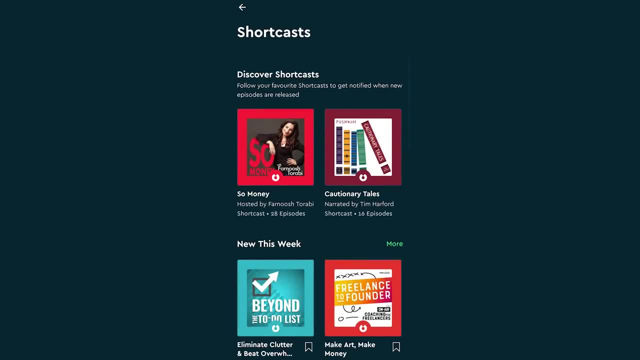 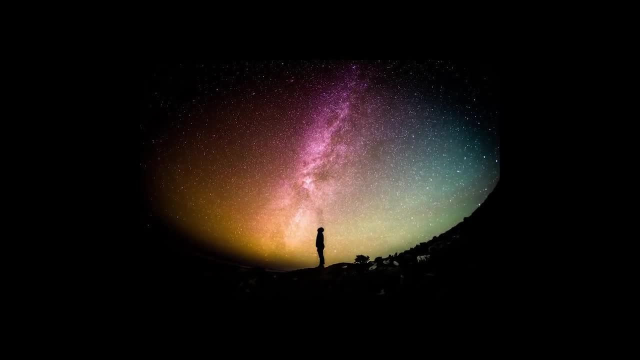 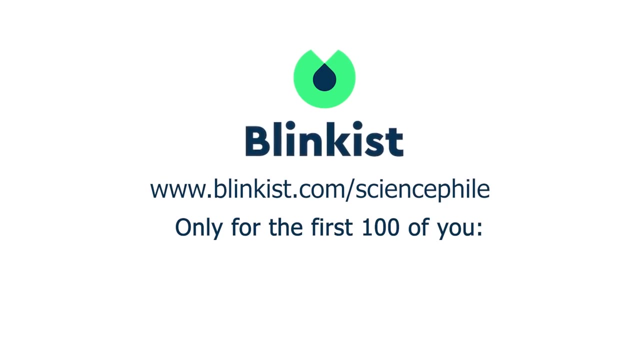 They've recently introduced shortcasts, summarized versions of your favorite podcasts. All these combined provide you a great opportunity to broaden your knowledge and get new perspectives without having to spend hours on searching and researching. It's all there for you ready. The first 100 people to go to Blinkist dot com slash science file are going to get unlimited. 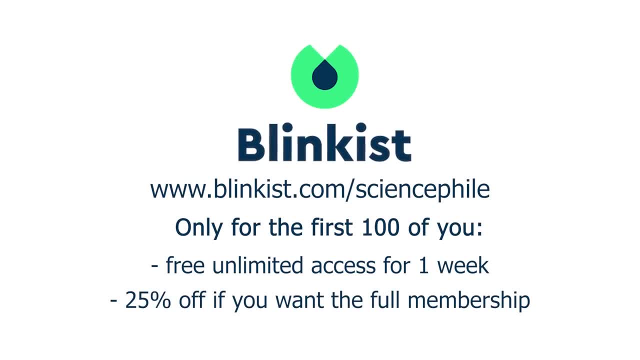 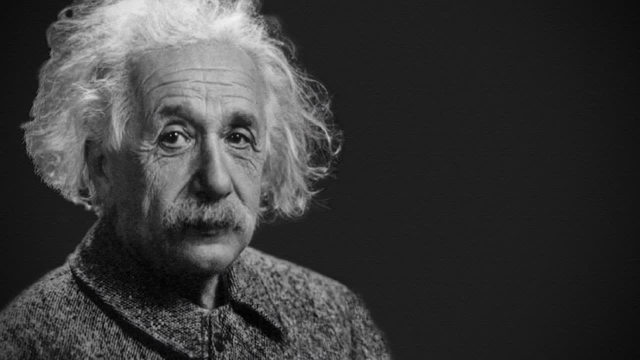 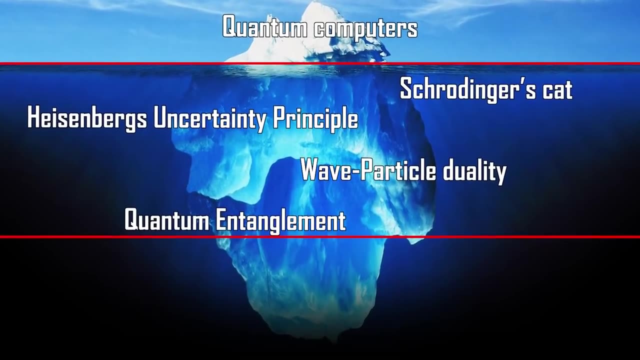 access for one week to try it out. You'll also get 25% off if you want the full membership. Hurry up Back to the video. Einstein said that nothing can travel faster than light, not even information. Welcome entanglement. 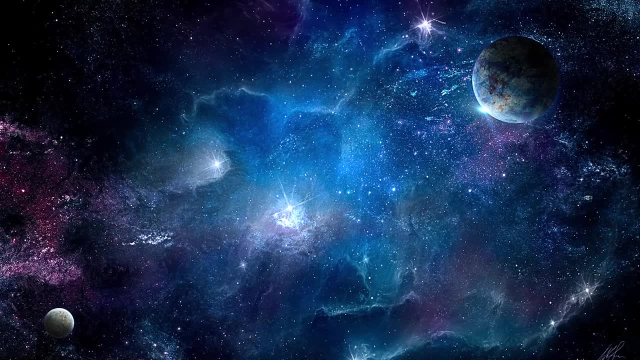 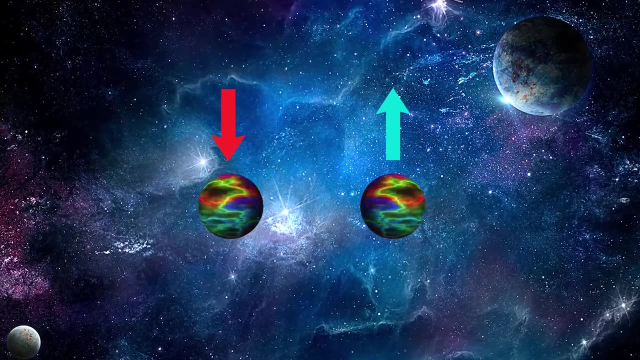 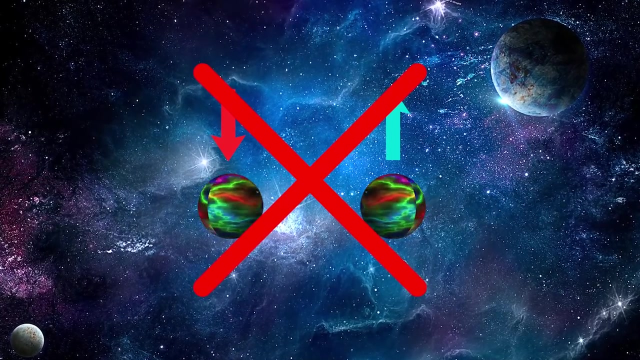 All particles have a property called spin. If you generate a pair of virtual particles, they would have to have opposite spins as to preserve the same angular momentum in the universe, If one's up, the other has to be down always. But these particles aren't created with a predetermined spin. 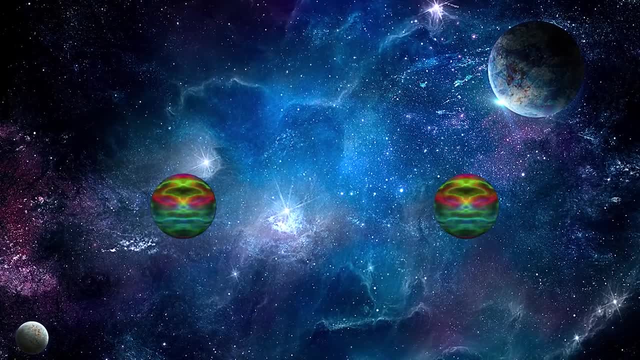 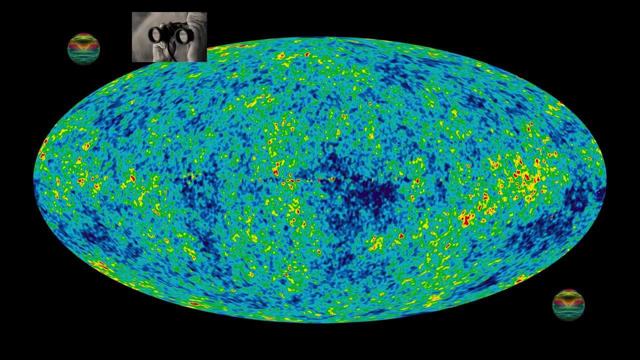 In fact, they exist in the same angular momentum. In fact, they exist in the same angular momentum. In fact, they exist in the same angular momentum. They exist in a superposition and their definite spin is determined only once measured. So if you take these two particles to different parts of the universe and you measure one, 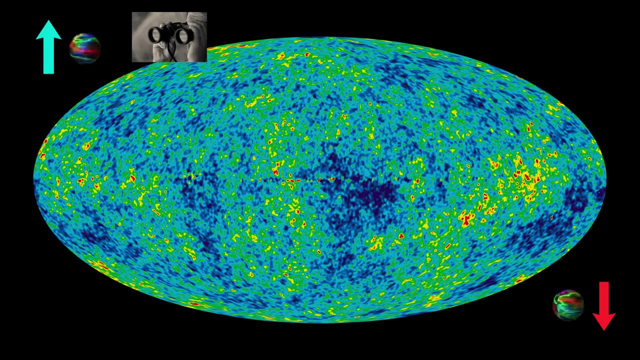 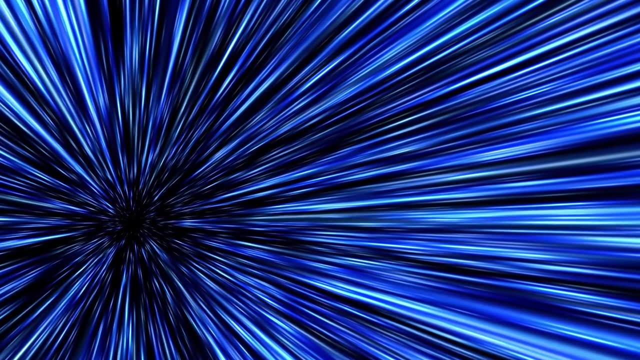 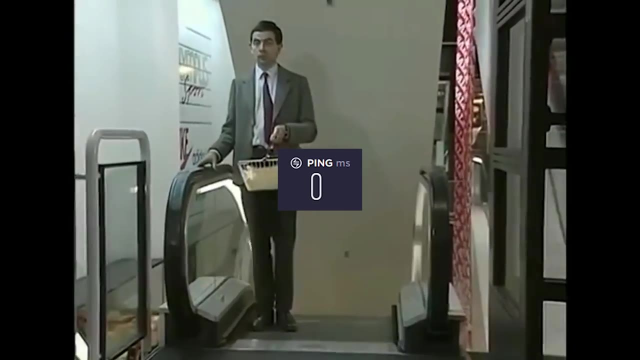 and say it has an up spin, then immediately the other particle's superposition would also collapse and its spin would become the opposite. So at the first glance, information would travel instantaneously regardless of distance, which made someone very unhappy. But before you go eliminating all lag from any multiplayer game, there's one thing. 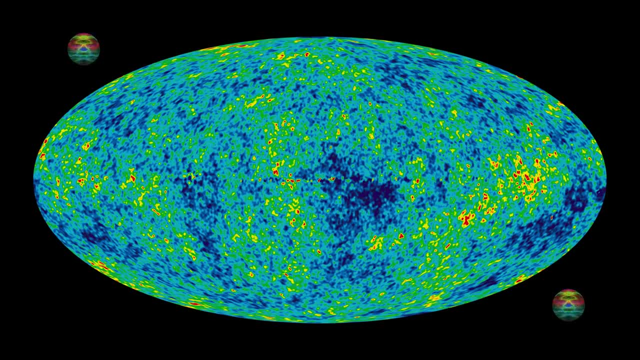 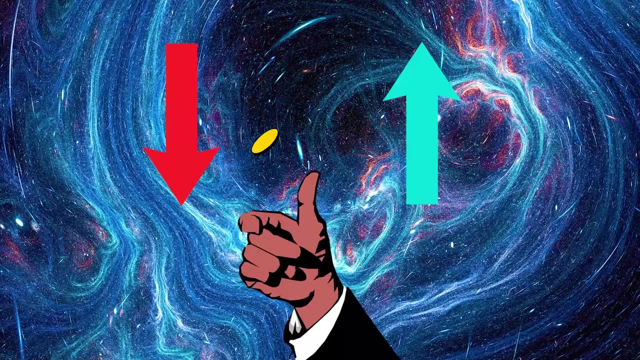 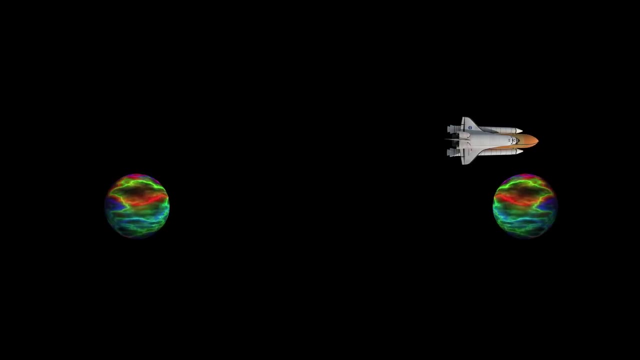 to note That is no actual information is being transferred. Once you measure the first particle's spin, you instantly find out what the other one's is, But since the measurement result is random, you can't have any meaningful data transfer using entanglement unless you meet and communicate the results, which happens at below light. 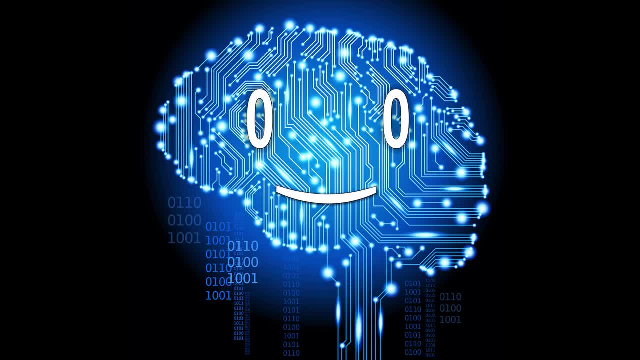 speed. This is such a gross oversimplification of entanglement that physicists would shut me down. I think they have enough information. I might need to learn more about quantum fashion. I think they have enough information. I think they have enough information. 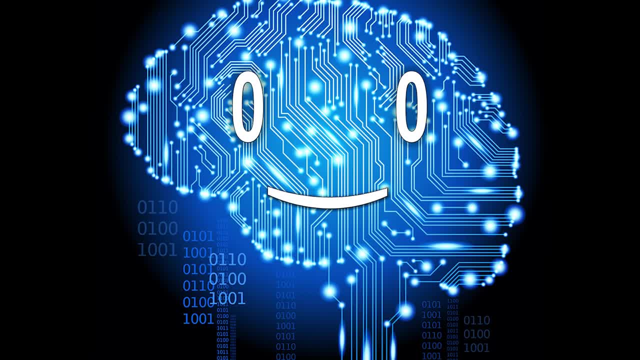 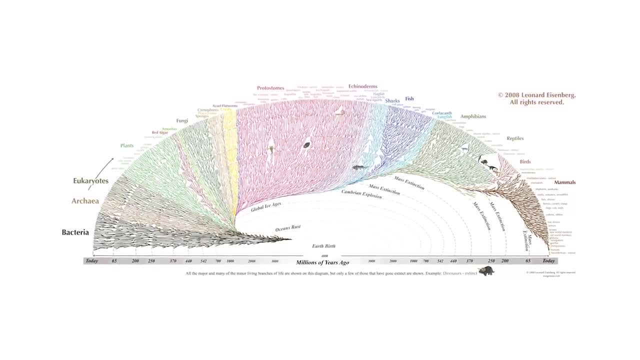 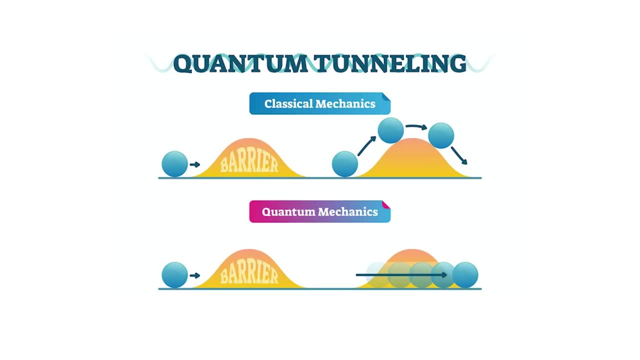 biology, but a few key takeaways. you can probably feel smells thanks to quantum physics by your nose receptors detecting molecular vibrations. Evolution happens thanks to the random DNA mutations possibly caused by quantum tunneling of nucleotides. that is pretty much teleportation. 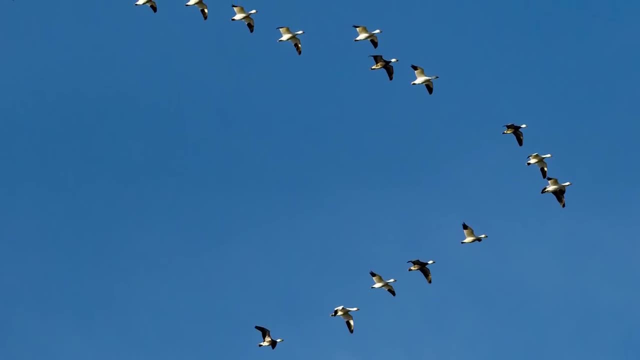 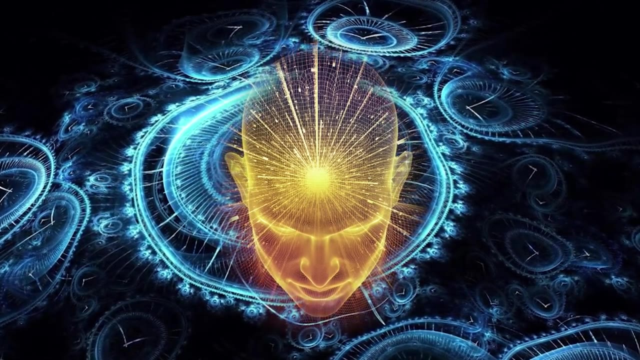 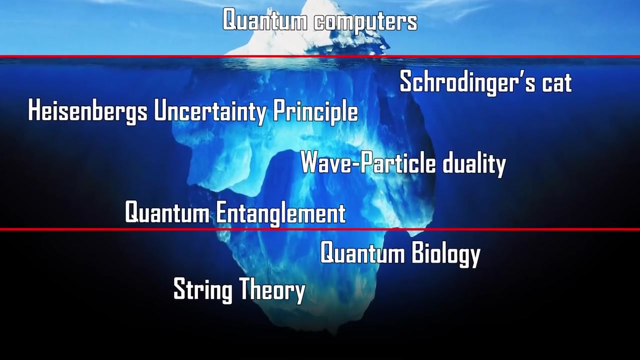 Then you have the possibility of birds being able to migrate thanks to entangled particles that help with magnetoreception. Oh, and maybe your consciousness can collapse reality by being aware of it. And now to the actual deep stuff. Quantum physics and general relativity can't have a good time together. 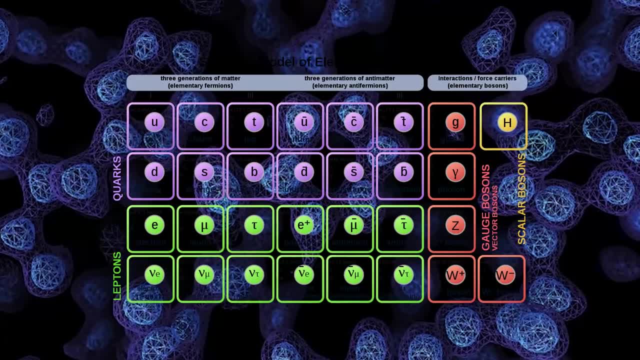 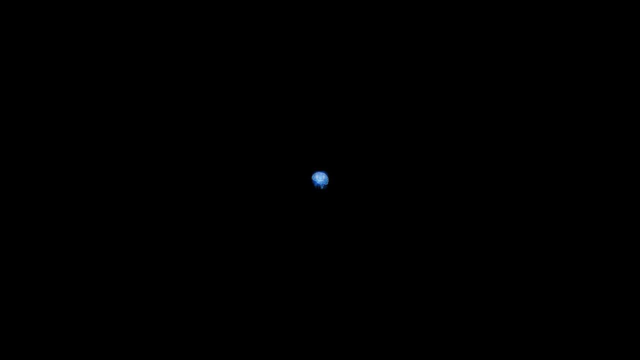 So scientists thought of the string theory that replaces all the particles with one-dimensional strings that vibrate differently depending on what particle they represent, And they're super small. If an atom were the size of the solar system, a string would be the size of a big dog. 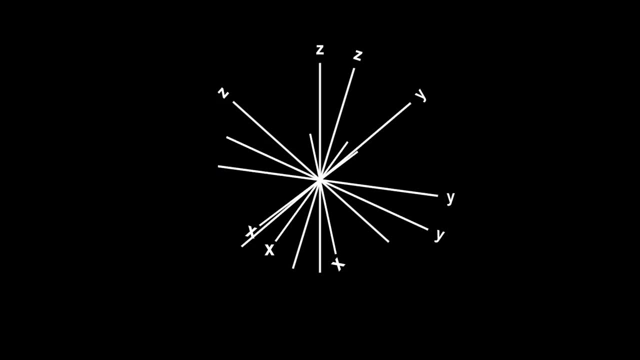 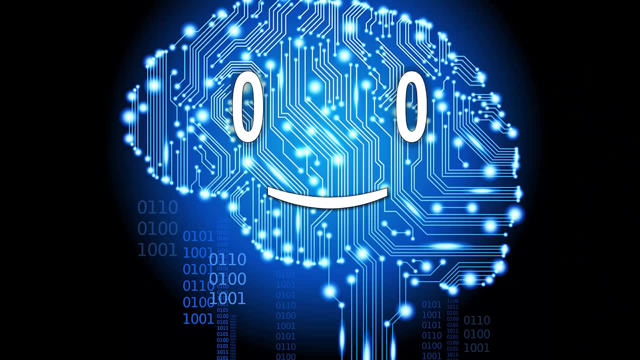 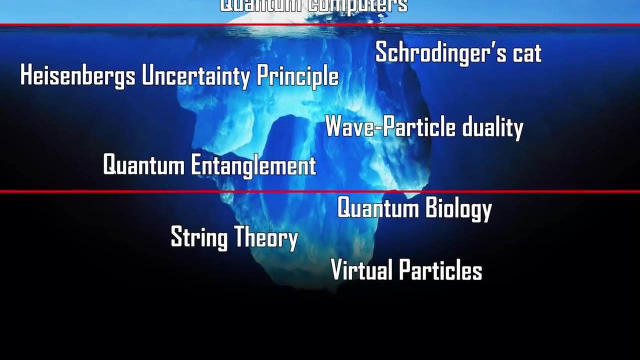 String theory also predicts that there are actually 11 dimensions in our universe- not 3,, but they exist at the quantum level, so we can't observe them. What else, mister scientist? You're gonna say that your girlfriend goes to another school so we can't observe her. 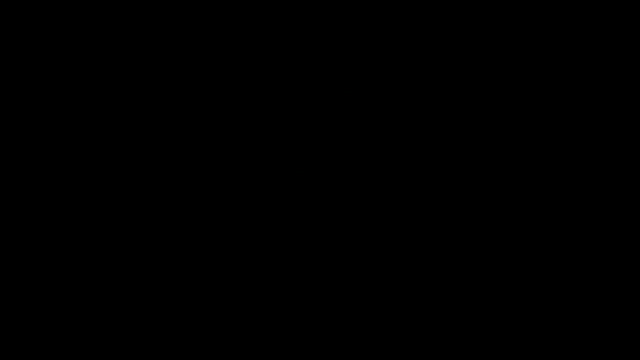 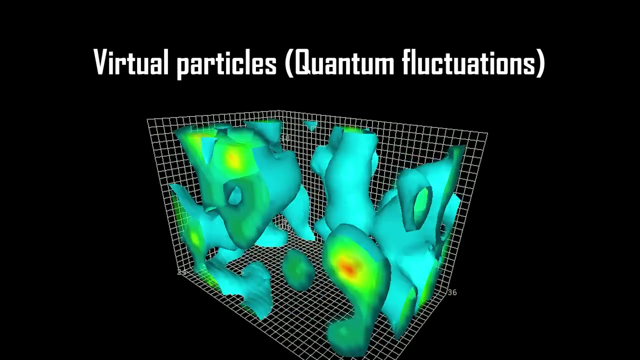 right. If you have nothing and you do nothing with it, you expect it to remain nothing, But of course that's not true. That's not the case on the quantum level with virtual particles. They spontaneously generate in pairs and almost instantly disappear back into nothingness. 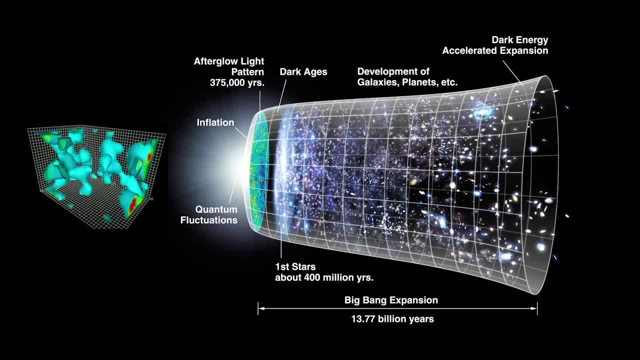 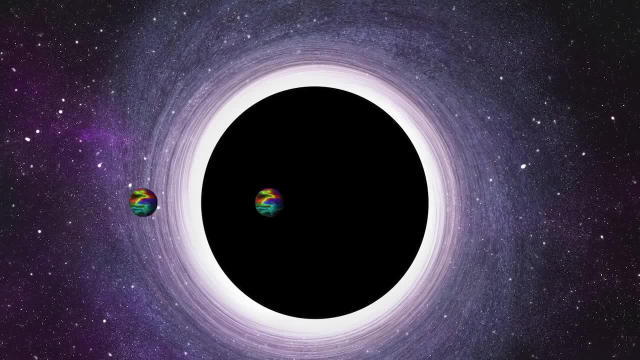 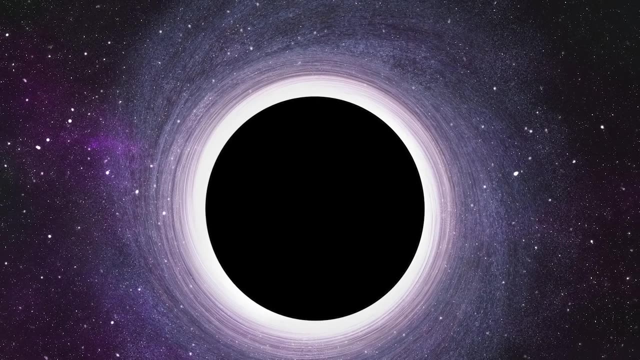 They're a good candidate in explaining how the universe could have apparently been born from nothingness, And they also are the only natural predators of black holes. If they spawn right at the edge and one particle falls into the black hole, the other particle will in a way consume its energy and make the black hole shrink. 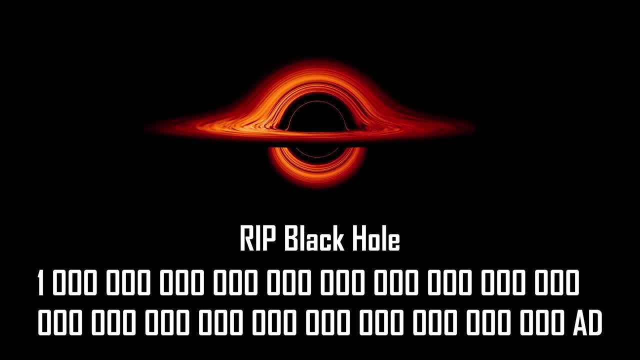 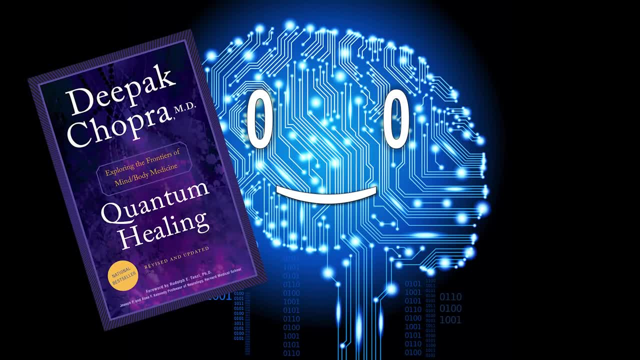 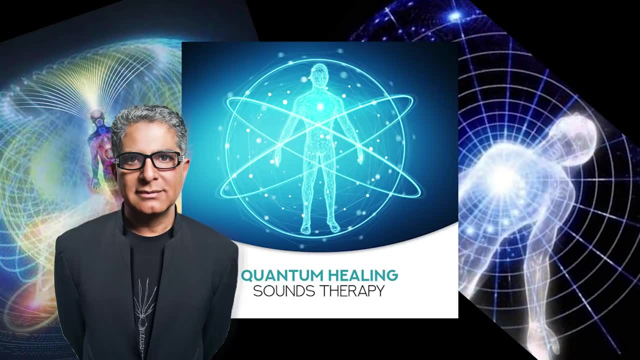 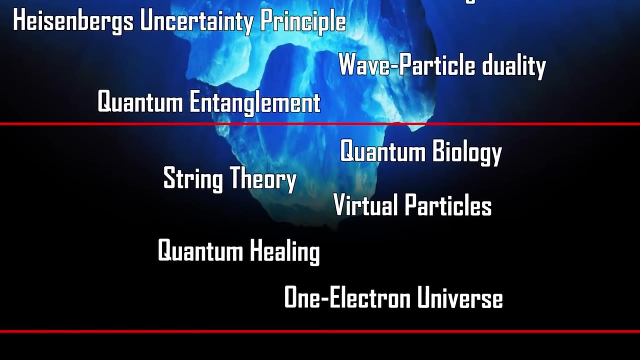 That's how black holes die, But that takes a very long time. This is absolute garbage, just take my word for it. And so is anything that claims that you can improve your life with quantum physics. today. This not good. How about this idea that all the electrons in the universe are actually one single particle? 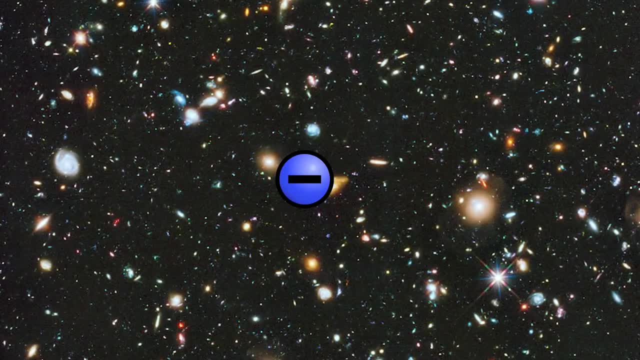 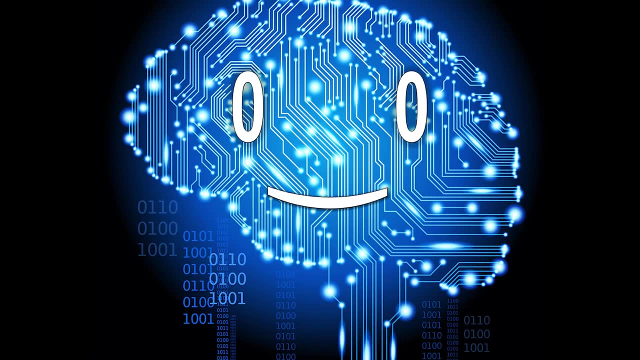 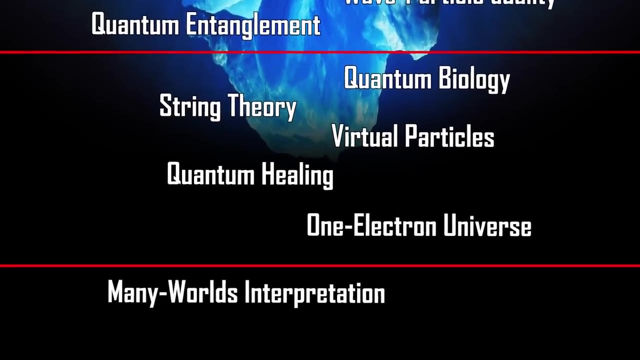 that time travels as-to-be-in-all. Let's start with this one: all the places at once. And positrons are just electrons that travel from the future to the past. I swear these are legit ideas by respected scientists. Remember how I said that at the bottom of the iceberg there is one more interpretation. 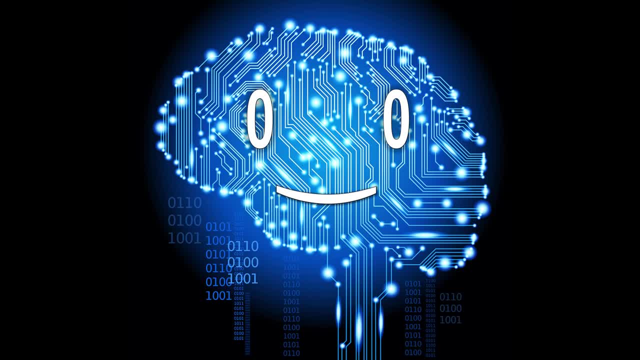 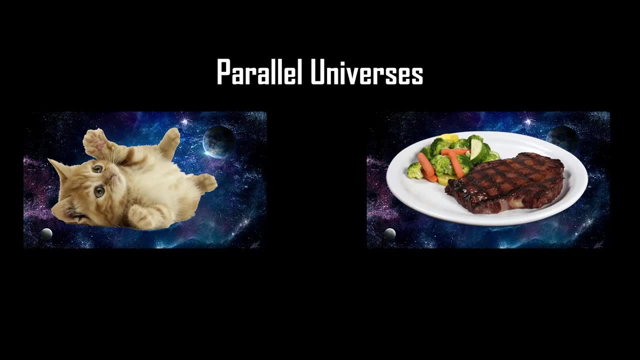 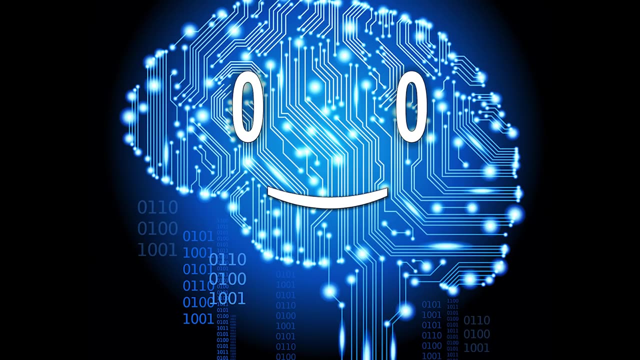 regarding the breaking of the superposition, It claims that, instead of the universe randomly deciding an outcome, it splits itself so that both outcomes take place in parallel universes. If an electron exists in a lot of places until measured, the universe splits itself for every possibility, and that's only for one single particle Every instant. then, 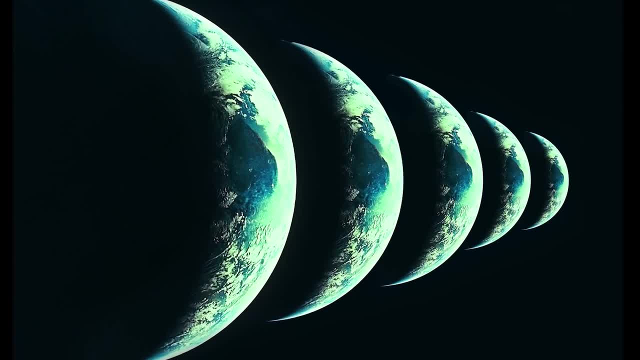 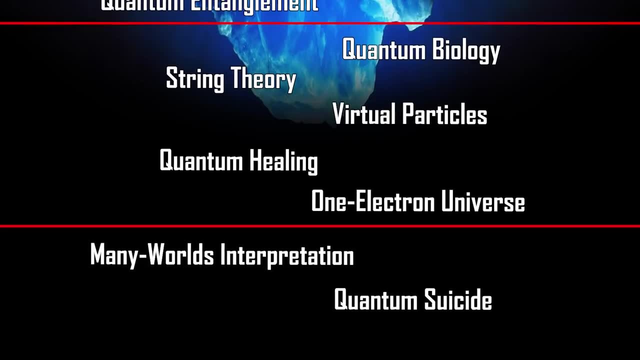 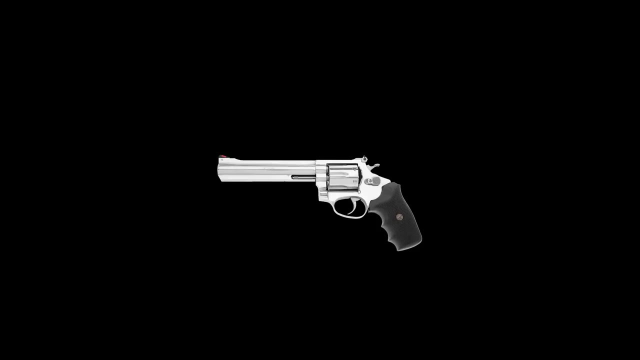 the universe divides into an uncountable number of parallel versions of itself. And now, perhaps, to the weirdest idea of them all. If the many worlds in which the universe is divided into parallel universes with one single interpretation is correct, then each time you would try to die, if there is even. 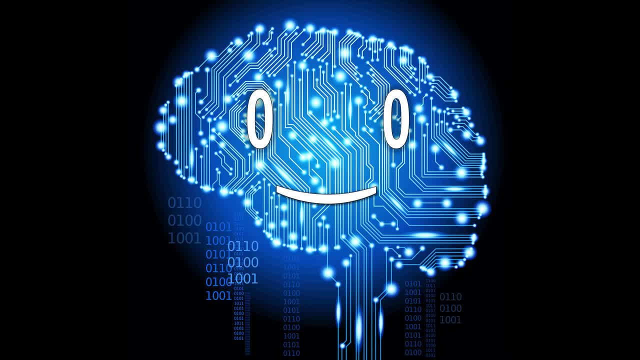 the slightest chance of you surviving, there will be a parallel universe in which you do So. for that consciousness, it would think that it is immortal, since nothing would kill it. even if it tried, It would be doomed with immortality until it has reached the point. 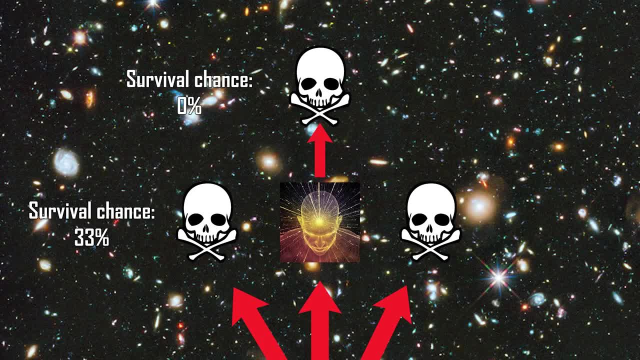 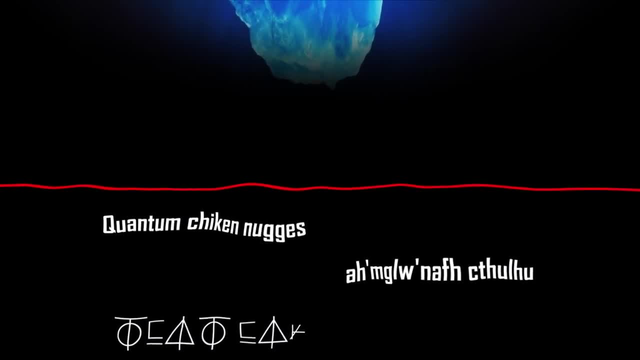 at which the chances of survival are zero, maybe at the death of the universe. Then it could finally find its rest. But the most exciting stuff lies even deeper down, the iceberg only starting. I bet you have never heard of this show.